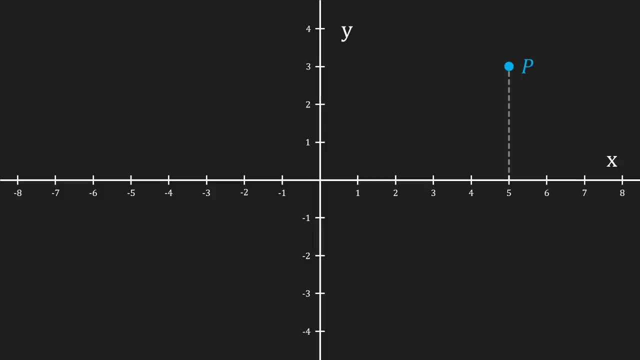 its position. We do that by tracing a line parallel to the y-axis onto the x-axis and a line parallel to the x-axis onto the y-axis. This gives us an x-coordinate of 5 and a y-coordinate of 3.. We note these between parentheses. 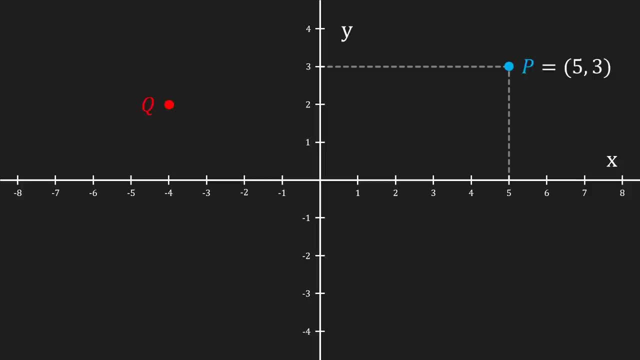 Just for fun, let's start with the x-coordinate. For fun, I'm going to add a point q and to calculate its coordinates. we do the exact same thing: We trace two lines and then we get an x-coordinate of negative 4 and a y-coordinate. 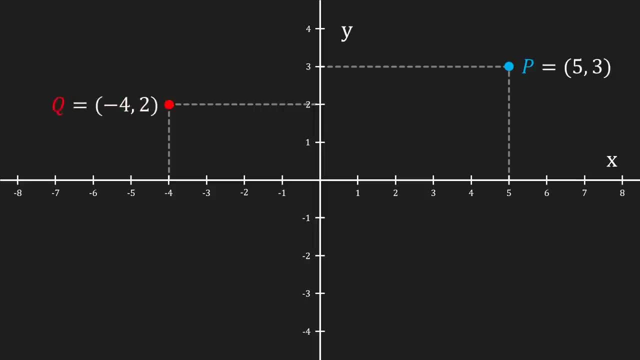 of 2.. Do note that we always write the x-coordinate first and then the y-coordinate. There's also a special point, and that is where the x and y-axis cross. We call that point the origin. We often give it the letter o, and its x and y-coordinates are 0.. Alright, now we are ready. 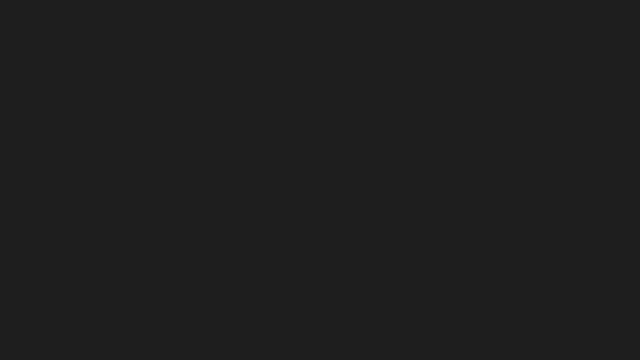 to move on to the next point, Let's start with the x-coordinate. In contrast to points, vectors do not have a position. We also don't use a point to represent them, but instead use an arrow. Vectors are defined by their length, which can become longer. 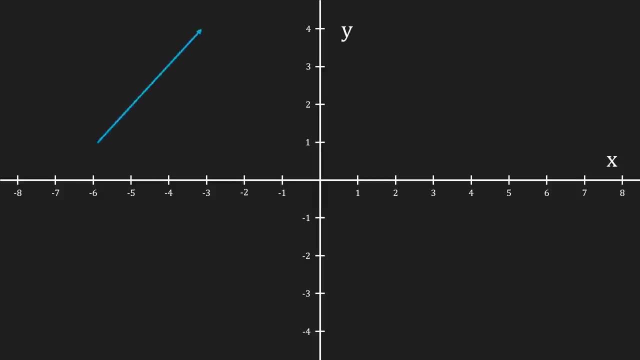 or shorter, and their direction, which is the way in which they point. Since they don't have a position, we can perfectly move the vector somewhere else, and it is still the same vector. I'm going to give this vector the letter a and the bar on top of it. 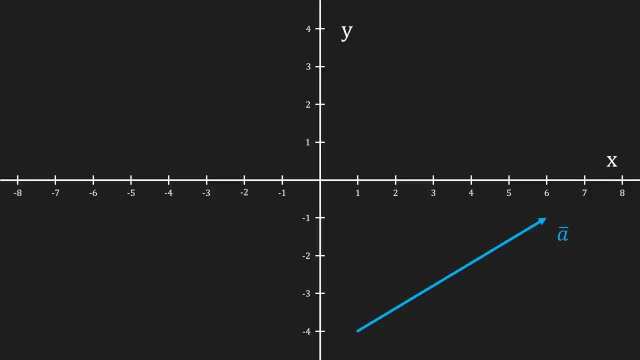 means that we are talking about a vector. To assign the x and y-components of a vector, we calculate how many steps the vector goes left or right and how many steps it goes up or down. In this case, the vector goes 5 steps to the right. Positive numbers indicate rightward motion. 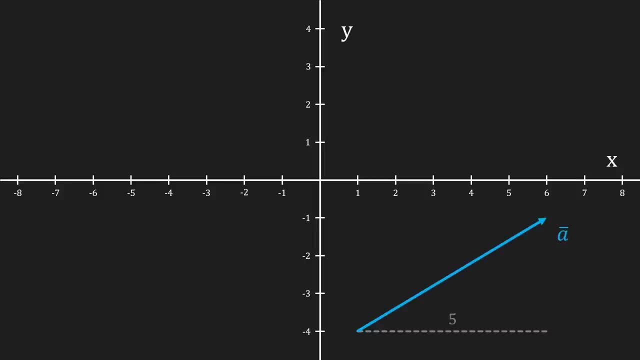 and negative numbers indicate leftward motion. The vector goes 3 steps up, and positive numbers indicate upward motion and negative numbers downward motion. The vector's components are divided between square brackets, like so, with the x-component on top and the y-component at the bottom. 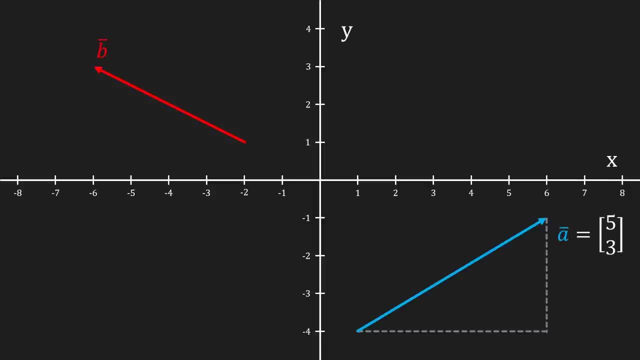 Just for fun, let's also add another vector, b. To calculate its components, we take 4 steps to the left, which gives us negative 4, and we take 2 steps up. We can then write its components once again between square brackets. As I said earlier, vectors don't have a position. 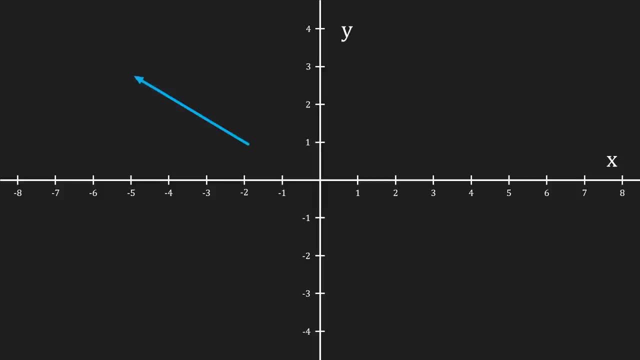 Vectors are defined by their length, which can become longer or shorter, and their direction, which is the way in which they point. Since they don't have a position, we can perfectly move the vector somewhere else, and it is still the same vector. I'm going to give this vector the letter a, and the bar on top of it we are talking about a vector. To assign the x and y-components of a vector, we calculate how many steps the vector goes left or right, and how many steps it goes up or down. In this case, the vector goes 5 steps to the right. Positive numbers indicate rightward motion, and negative numbers indicate leftward motion. The vector goes 3 steps up, and positive numbers indicate upward motion, and negative numbers downward motion. The vector's components are written between square brackets like so, with the x-component on top and the y-component at the bottom. 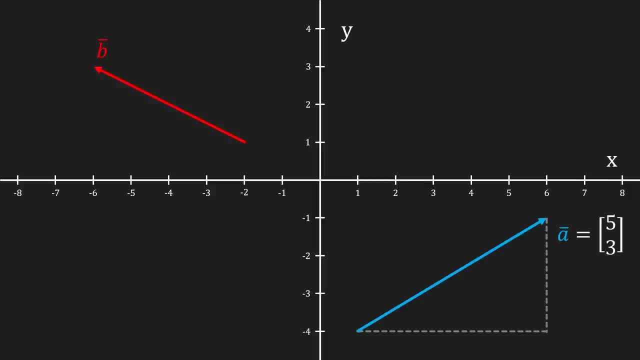 Just for fun, let's also add another vector, b. To calculate its components, we take 4 steps to the left, which gives us negative 4, and we take 2 steps up. We can then write these components once again between square brackets. As I said earlier, vectors do not have a position. However, if we assume that the tail of a vector is sitting at the origin, then we can think of a vector as being a point. Let's quickly have a word about notation. This is a two-dimensional vector. 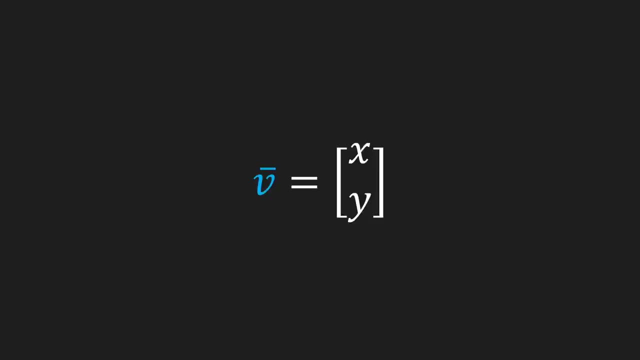 We write the x and y components between the square brackets. For a three-dimensional vector, we can add a z-component, and we would also add a z-axis, which would point outside of the screen. We can expand this vector even further by adding a w-component. Now you might be thinking, four-dimensional vectors? Wait, what? Well, we'll talk about that in the video about matrices. 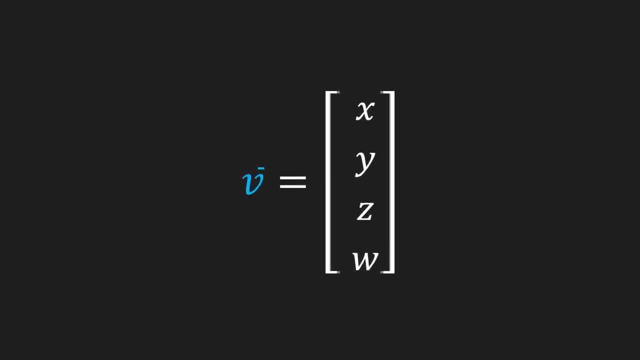 There's one last change I'm going to make here, and that is that I'm going to write these components as the subscript of the vector's name. 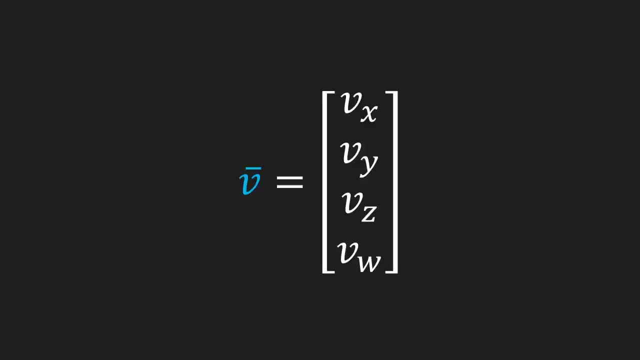 The reason why we do that is to not cause any confusion when we have multiple vectors. Finally, we can generalize this to n-dimensional vectors. We do that by not using x, y, z, and w, but just counting the components from 1 up to n. 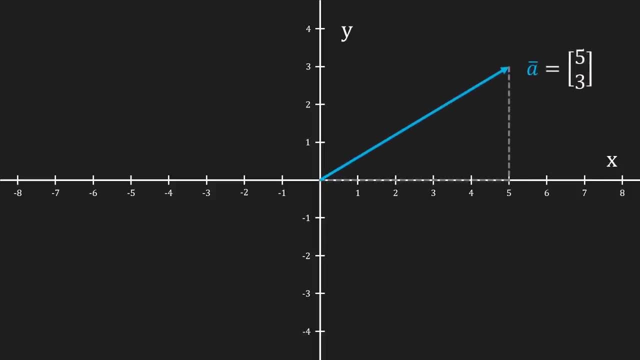 However, if we assume that the tail of a vector is sitting at the origin, then we can think of a vector as being a point. Let's quickly have a word about notation. This is a two-dimensional vector. We write the x and y components between the square brackets. 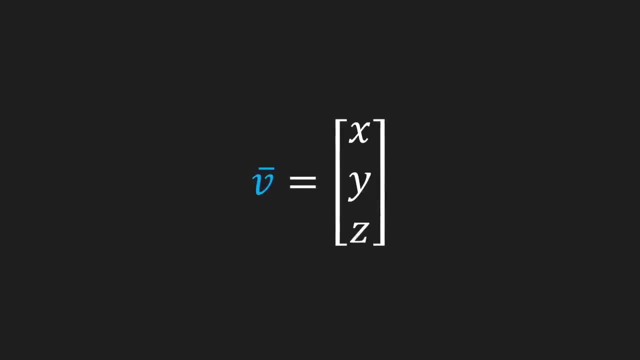 For a three-dimensional vector, we can add a z-component and we would also add a z-axis which would point outside of the screen. We can expand this vector even further by adding a w-component. Now you might be thinking four-dimensional vectors. 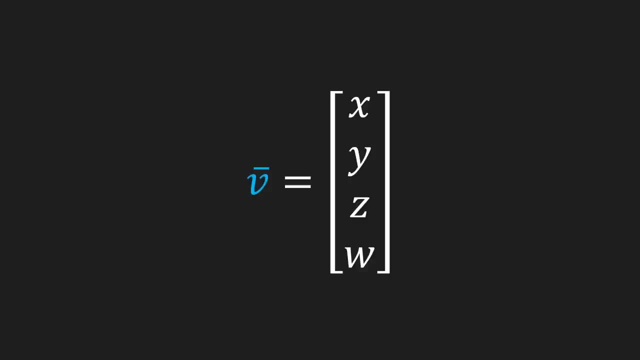 Wait, what Well? we'll talk about that in the video about matrices. There's one last change I'm going to make here, and that is that I'm going to write these components as the subscript of the vector's name. The reason why we do that is to not cause any confusion when we have multiple vectors. 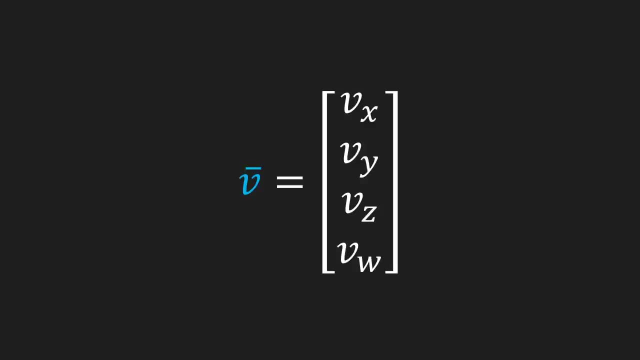 Finally, we can generalize this to n-dimensional vectors. We do that by not using x, y, z and w, but just counting the components from 1 up to n, Where n is the dimension of our vector. Alright, let's now move on to scalar operations. 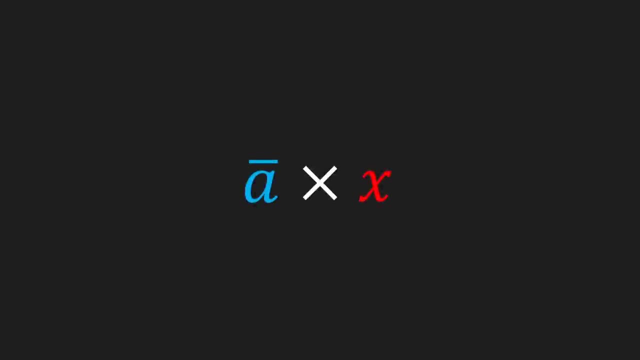 Scalar operations are just operations between a vector and a number. X is the number and it's also called a scalar, but more on that later. The operation could be a multiplication or a division. I'm going to continue to explain scalar multiplication, but scalar division is completely analogous. 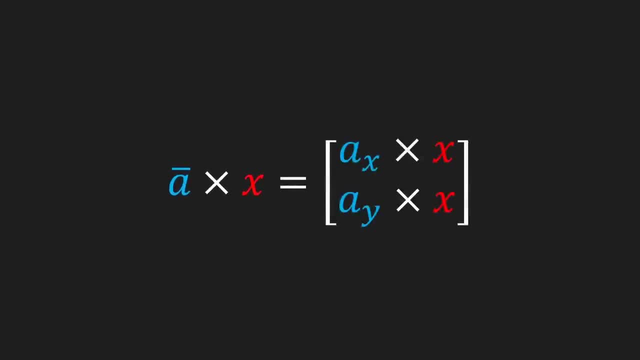 To multiply a vector with a scalar. we just multiply every component of that vector with the scalar. As an example, I'm going to take a vector a and an x value. We can now fill in these values in our equation and calculate the result of a times x. 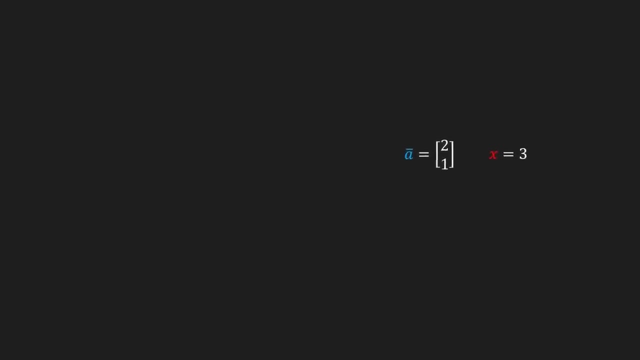 To clarify these numbers, I'm going to visualize vector a, and the result of its multiplication with x would be a new vector that is 3 times longer. In other words, this new vector is scaled by a vector of 2.. So the result of this new vector is 3 times longer. 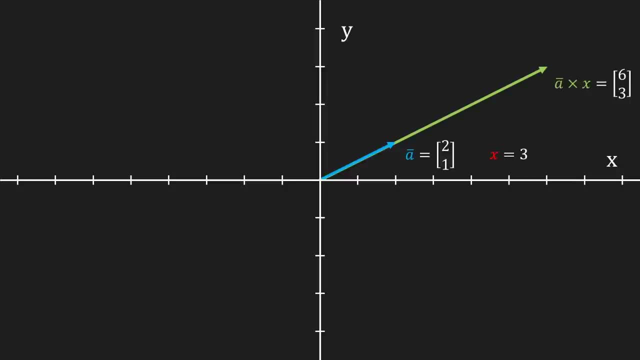 And that is why we call x a scalar For completeness. if we would have divided by x, we would get a vector that is 3 times shorter. There's a special case in which we multiply with an x value of negative 1.. 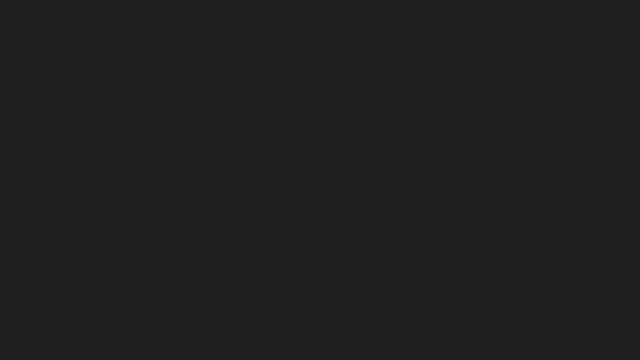 Where n is the dimension of our vector. Alright, let's now move on to scalar operations. 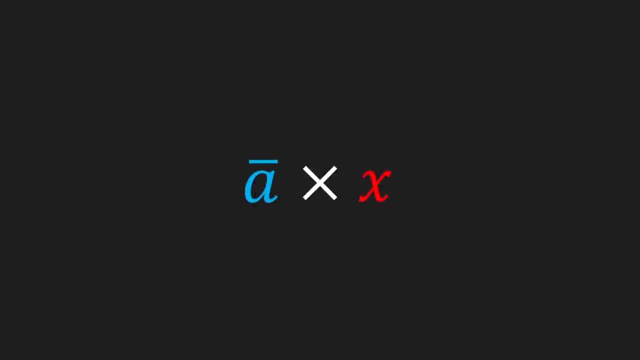 Scalar operations are just operations between a vector and a number. X is the number, and it's also called a scalar, but more on that later. The operation could be a multiplication or a division. 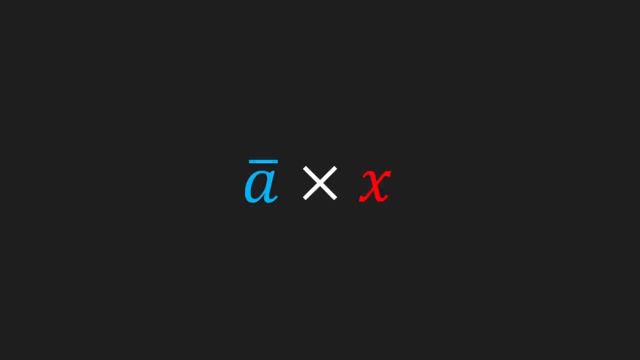 I'm going to continue to explain scalar multiplication, but scalar division is completely analogous. 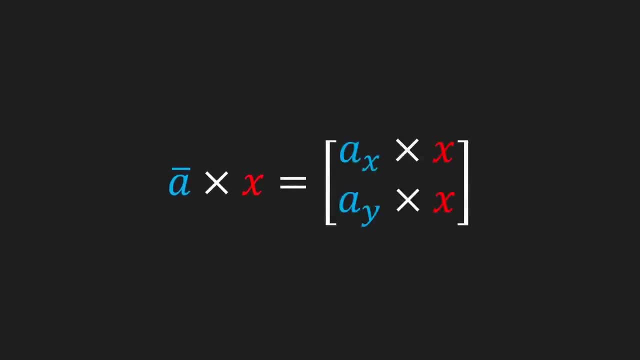 To multiply a vector with a scalar, we just multiply every component of that vector with the scalar. As an example, I'm going to take a vector a and an x value. We can now fill in these values in our equation, and calculate the result of a times x. To clarify these numbers, I'm going to visualize vector a, and the result of its multiplication with x would be a new vector that is 3 times longer. In other words, this new vector is scaled by a vector of 2. So, the result of this new vector is 3 times longer. And that is why we call x a scalar. 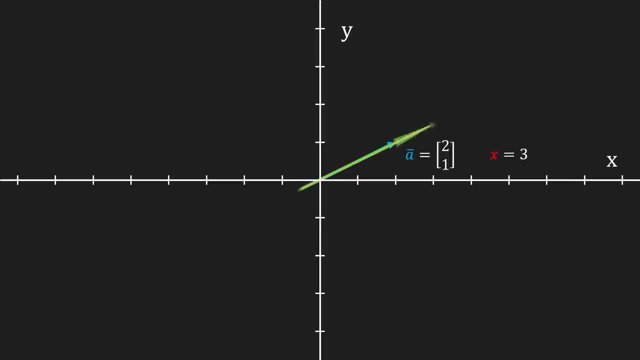 For completeness, if we would have divided by x, we would get a vector that is 3 times shorter. There's a special case in which we multiply with an x value of negative 1. As you can see, in this case, the vector's components have become the opposite, and the vector itself also points in the opposite direction of the original vector. 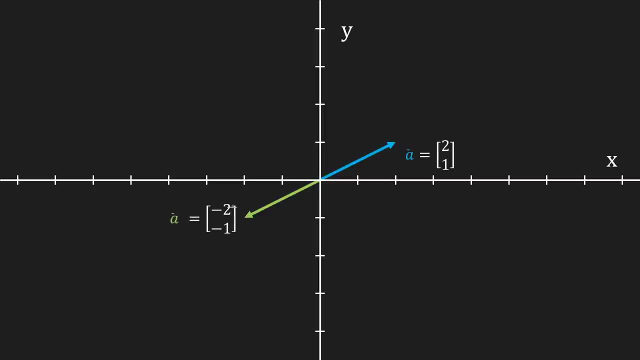 To simplify this, we just say that the green vector is just negative a. 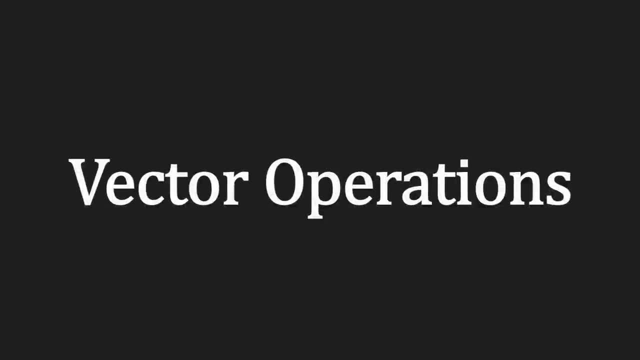 Now that we know what scalar operations are, we can now calculate the result of a scalar. Let's move on to vector operations, which are operations between two vectors. This could be either an addition or a subtraction. 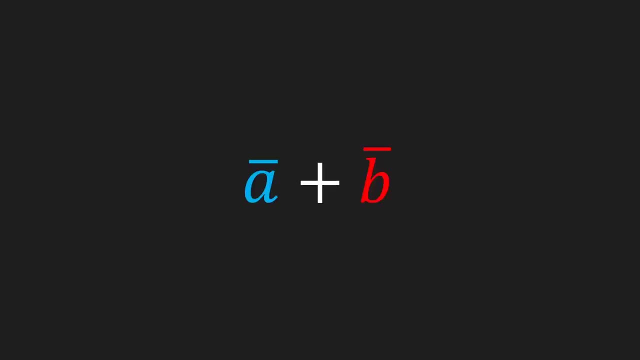 I'm going to continue to explain vector addition, but once again, vector subtraction is completely analogous. 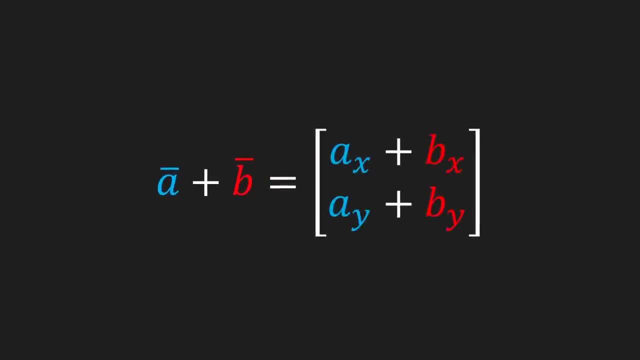 To calculate the sum of two vectors, we just calculate the sum of their x components, and the sum of their y components. 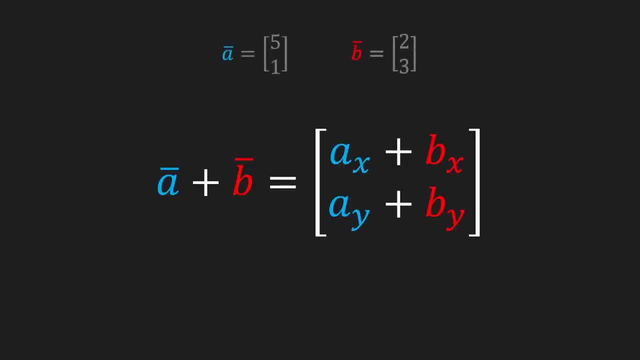 As an example, I'm going to take two vectors, a and b, I'll fill in their values in our formula. 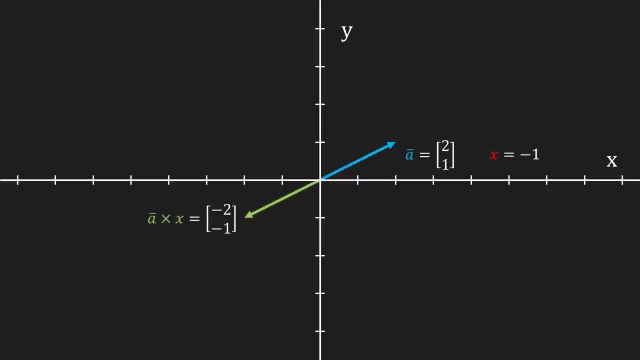 As you can see, in this case the vector's components have become the opposite and the vector itself also points in the opposite direction of the original vector. To simplify this, we just say that the green vector is just negative a. Now that we know what scalar operations are, we can now calculate the result of a scalar 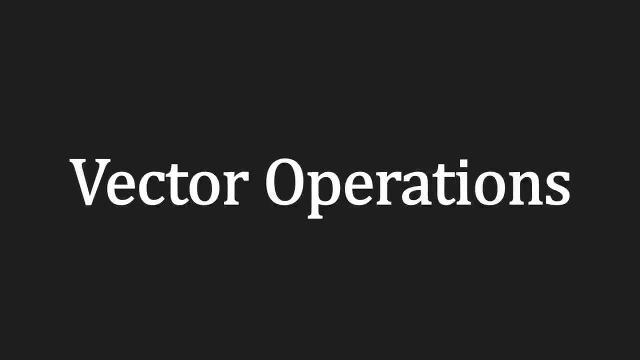 Let's move on to vector operations, which are operations between two vectors. This could be either an addition or a subtraction. I'm going to continue to explain vector addition, but once again, vector subtraction is completely analogous. To calculate the sum of two vectors, we just calculate the sum of their x components and 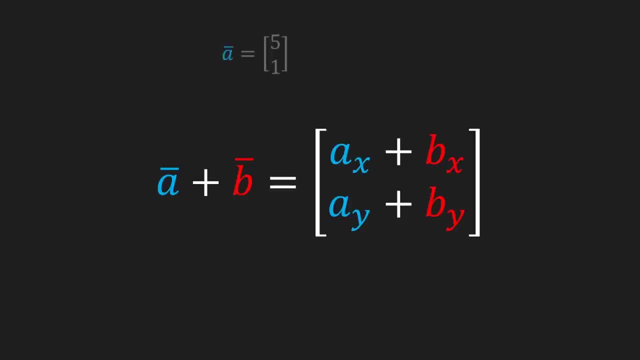 the sum of their y components. As an example, I'm going to take two vectors, a and b. I'll fill in their values in our formula. Now we can calculate the sum of a and b. That's all great and everything, but let's actually draw these vectors and visualize. 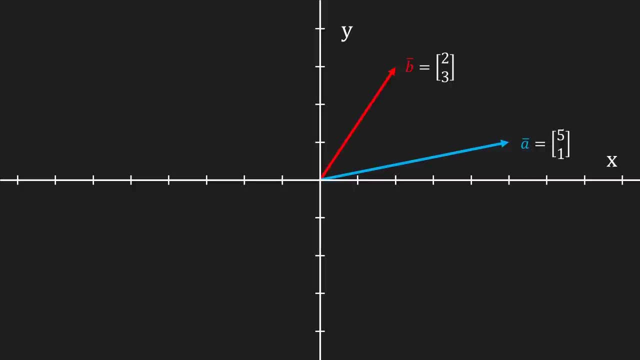 the result of their addition. To visualize that I'm going to move vector b's tail to the tip of vector a. The result of their addition is then a new vector that starts at the tail of vector a and ends at the tip of vector b. 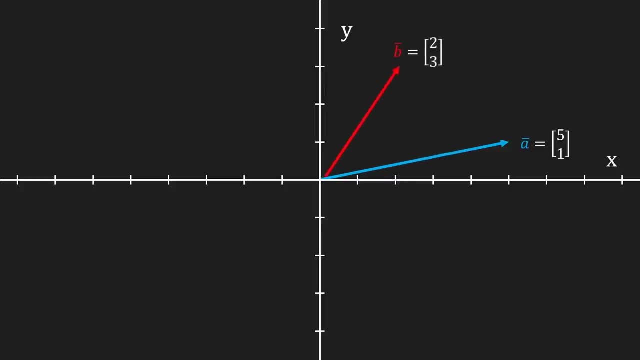 For completeness, let's also talk about how subtracting vectors would look. In that case, we would get a vector that goes to the top of vector a and ends at the top of vector b. Now why is this useful? As I said earlier, we can think of vectors as being points if their tail is sitting. 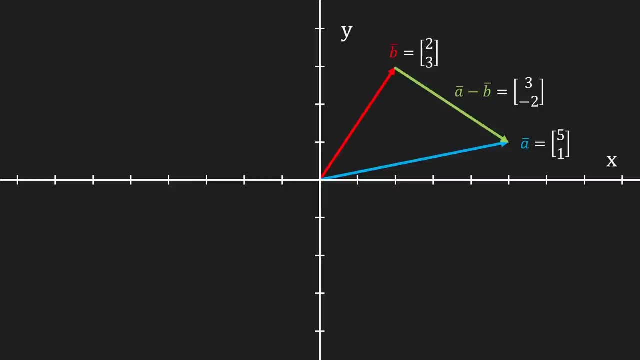 at the origin And, lucky for us, vector a and b's tail are sitting at the origin, so we can think of them as points. And now you see that we can use vector subtraction to calculate a vector from one point to the other. 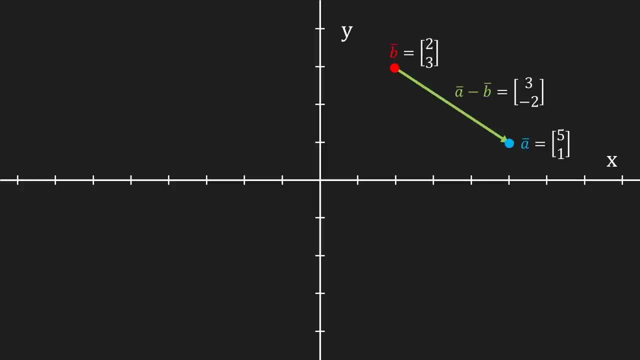 What's even more interesting is that if we calculate the length of the vector, we can know the distance between these two points. Talking of length, let's actually discuss the length of a vector. We also refer to it as the magnitude or norm. 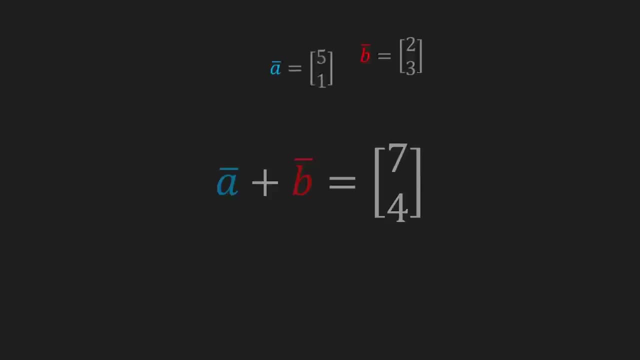 Now we can calculate the sum of a and b. That's all great and everything, but let's actually draw these vectors and visualize the result of their addition. 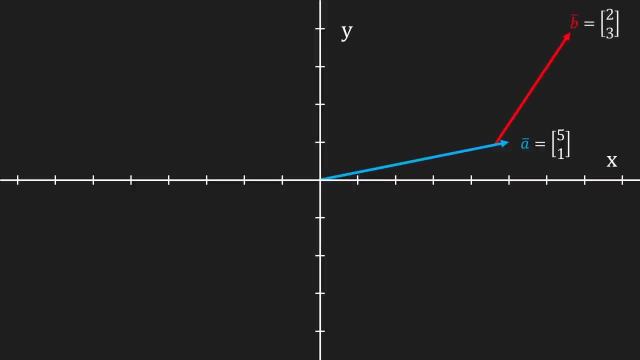 To visualize that, I'm going to move vector b's tail to the tip of vector a. The result of their addition is then a new vector that starts at the tail of vector a and ends at the tip of vector b. 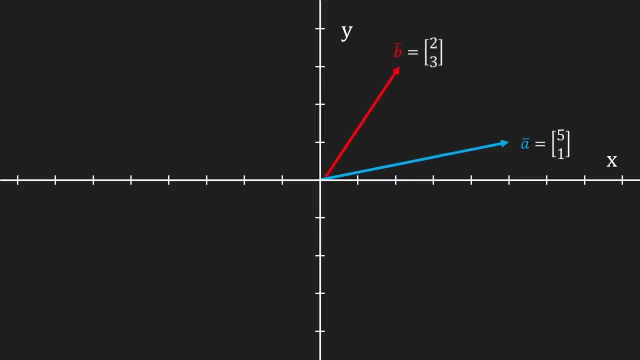 For completeness, let's also talk about how subtracting vectors would look. In that case, we would get a vector that goes to the top of vector a, and ends at the top of vector b. 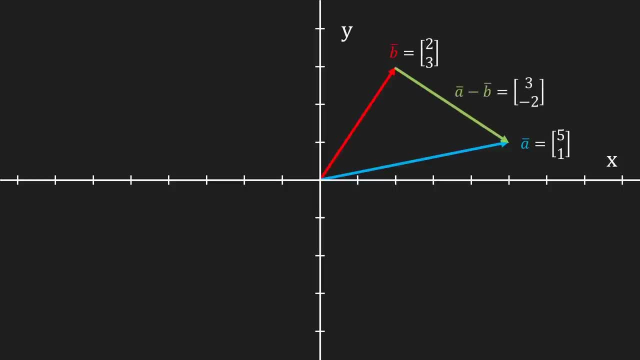 Now, why is this useful? As I said earlier, we can think of vectors as being points, if their tail is sitting at the origin. 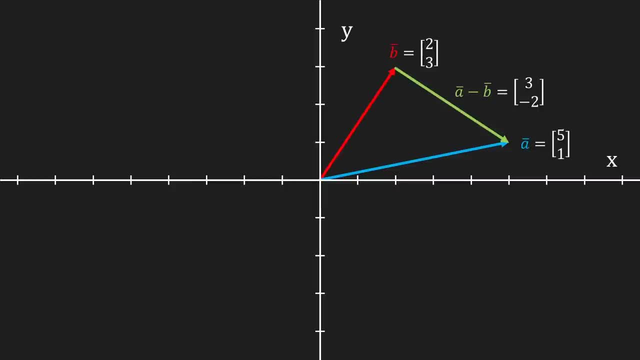 And lucky for us, vector a and b's tail are sitting at the origin, so we can think of them as points. 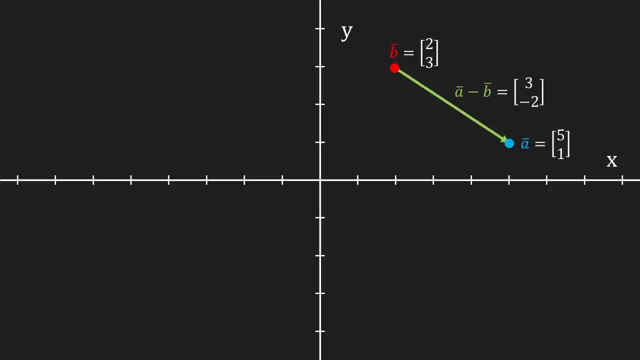 And now you see that we can use vector subtraction to calculate a vector from one point to the other. 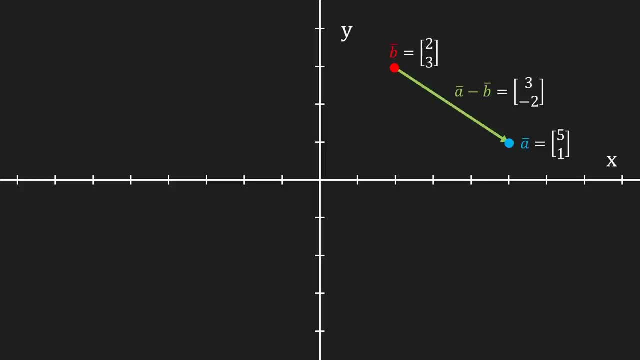 What's even more interesting is that if we calculate the length of the vector, we can know the distance between these two points. 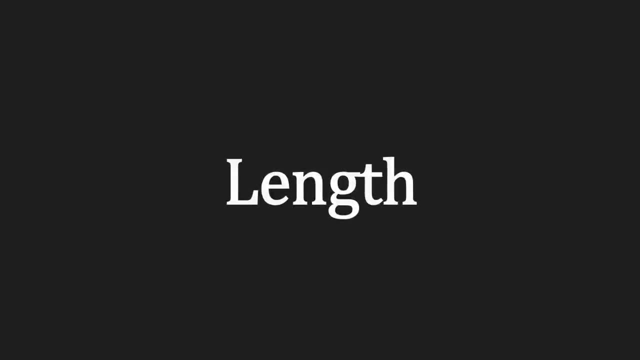 Talking of length, let's actually discuss the length of a vector. We also refer to it as the magnitude, or norm. 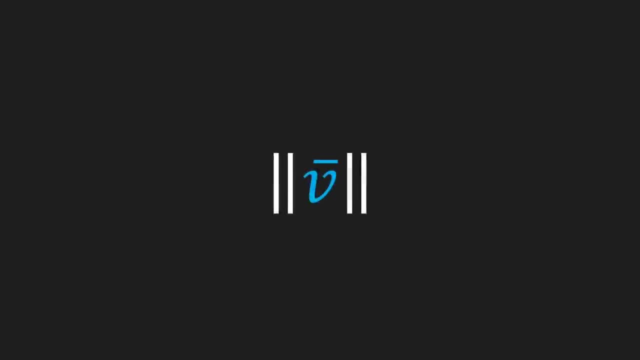 We represent it by writing these two vertical bars on either side of our vector. 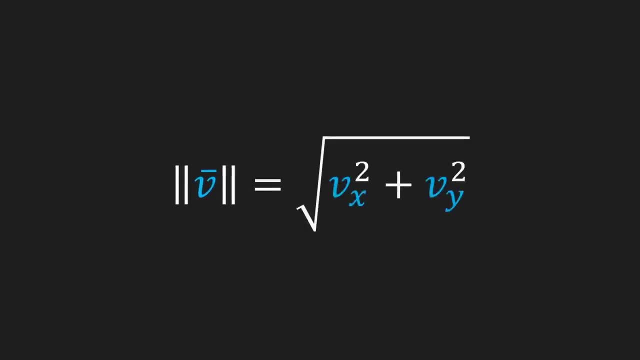 And in two dimensions, the length of a vector is defined by this formula. 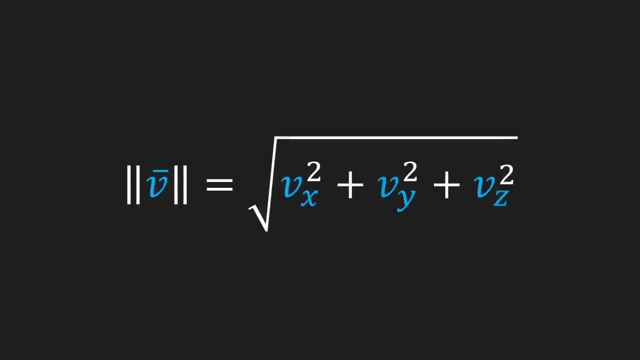 We can extend that to three dimensions, and even write a version for the generic n-dimensional vector. 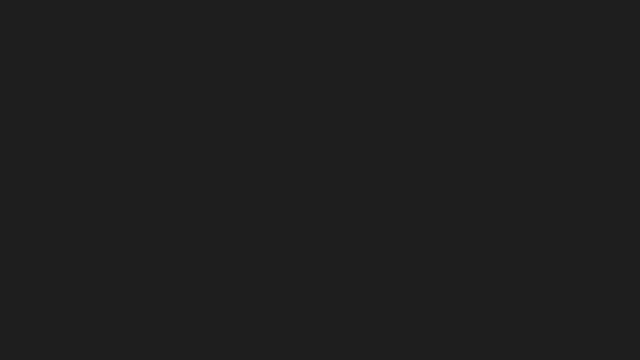 To understand how that formula works, we're gonna take our beloved coordinate system, and take a random vector, in this case vector v. Then I'm gonna draw a triangle beneath the vector, and do notice that I could have perfectly drawn it on top, it's just that I like to draw it beneath it. This triangle is a right-angled triangle. The width of that triangle is the vector's x-component, the height of that triangle is the vector's y-component, and then the hypotenuse, or tilted side of the triangle. 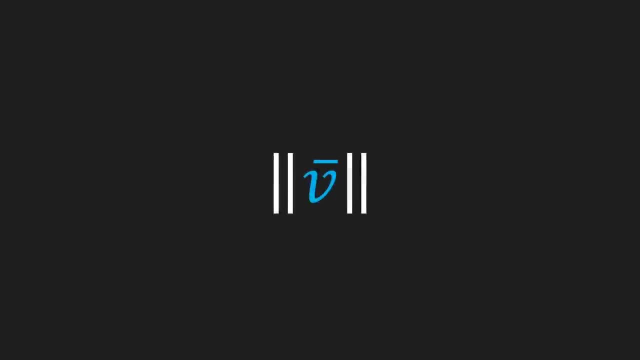 We represent it by writing these two vertical bars on either side of our vector And in two dimensions. the length of a vector is defined by this formula. We can extend that to three dimensions and even write a version for the generic n-dimensional vector. 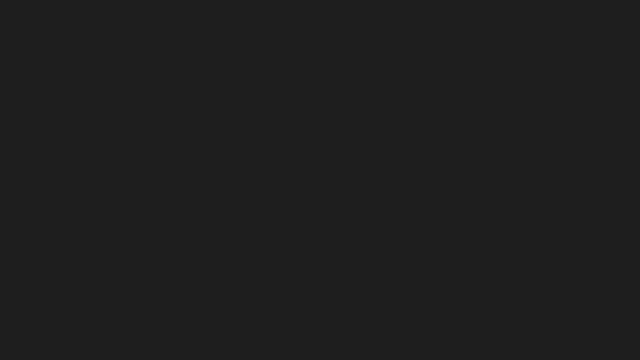 To understand how that formula works, we're gonna take our beloved coordinate system and take a random vector, in this case vector v. Then I'm gonna draw a triangle beneath the vector. and do notice that I could have perfectly drawn it on top, it's just that I like to draw it beneath it. 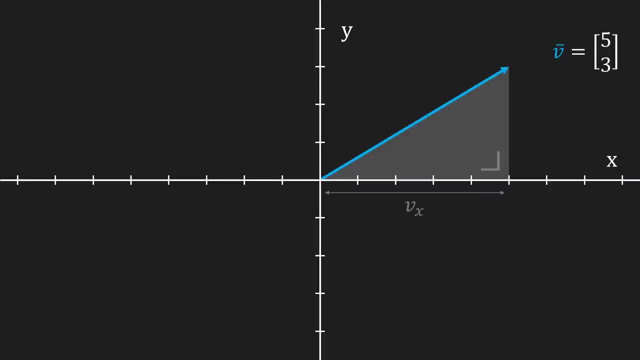 This triangle is a right-angled triangle. The width of that triangle is the vector's x-component, the height of that triangle is the vector's y-component, and then the hypotenuse or tilted side of the triangle. At this point we've got a right-angled triangle of which we know the width and the height. 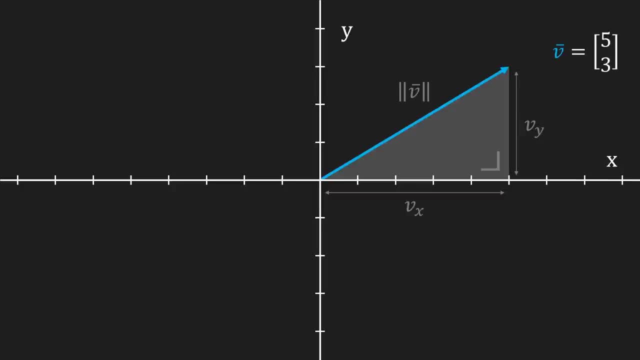 and we're looking for the length of its hypotenuse. And, lucky for us, there's been a famous mathematician called Pythagoras who came up with the Pythagoras theorem: a squared plus b squared equals c squared, where a and b are the width and height. 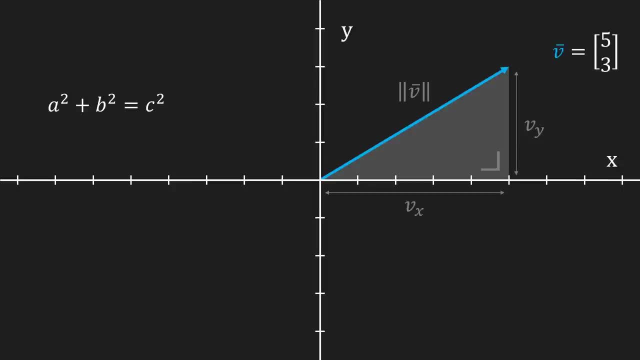 of a right-angled triangle and c is the length of its hypotenuse. We can now replace a, b and c with our vector's components. We can now replace a, b and c with our vector's components. We can now replace a, b and c with our vector's components and the vector's length. 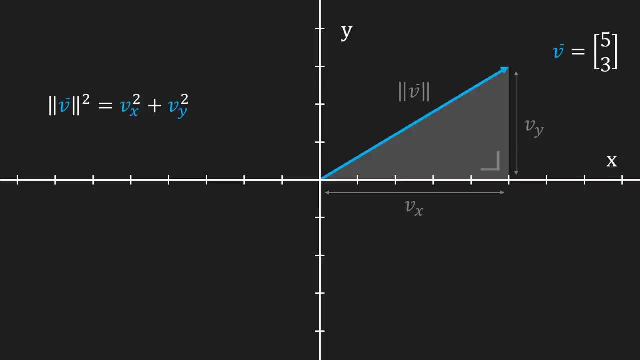 We'll swap the left and right side of that equation. we'll take the square root of either side of the equation and now we've got our expression for the length of a two-dimensional vector. If we fill in the components of that vector, in this case, we can calculate that this vector's 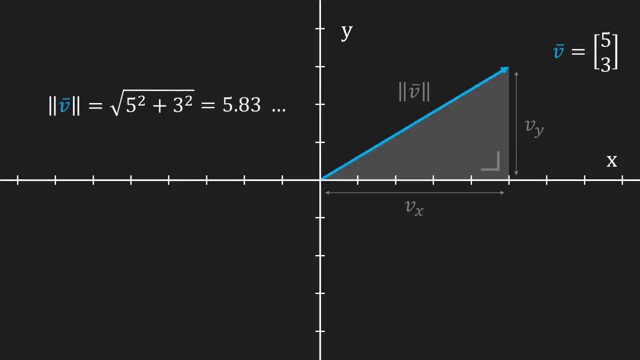 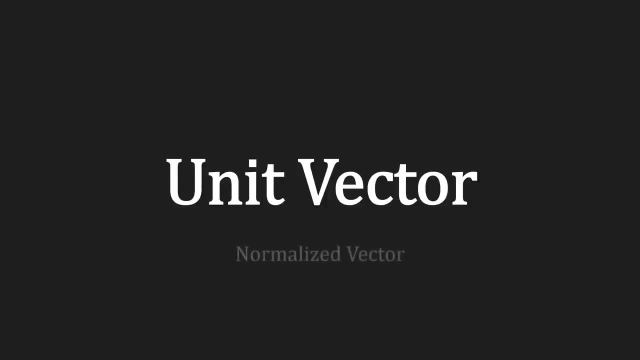 length is equal to 5.83 and a bit. Concerning a vector's length, there is a special case, which we call a unit vector. It's also referred to as a normalized vector. A normalized vector is a vector with a hat on top of it and a normalized or unit vector. 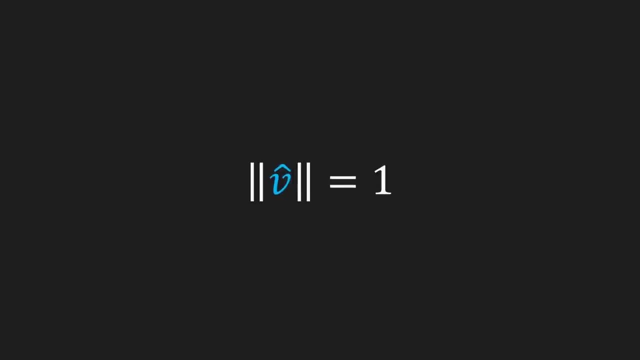 is nothing more than a vector with a length of 1.. In fact, we can take any arbitrary vector, divide it by its length, and then the result will be a vector that points in the same direction as the original vector, but that has a length. 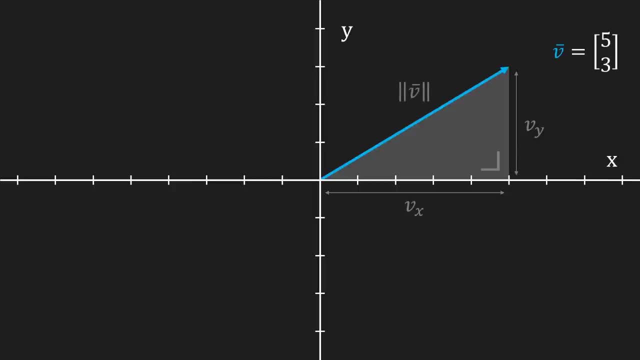 At this point, we've got a right-angled triangle, of which we know the width and the height, and we're looking for the length of its hypotenuse. 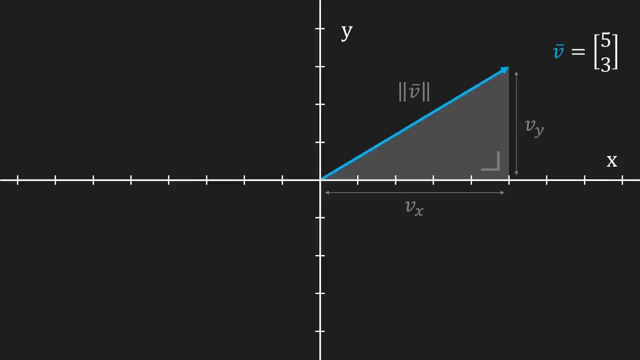 And lucky for us, there's been a famous mathematician called Pythagoras, who came up with the Pythagoras theorem, a squared plus b squared equals c squared, where a and b are the width and height 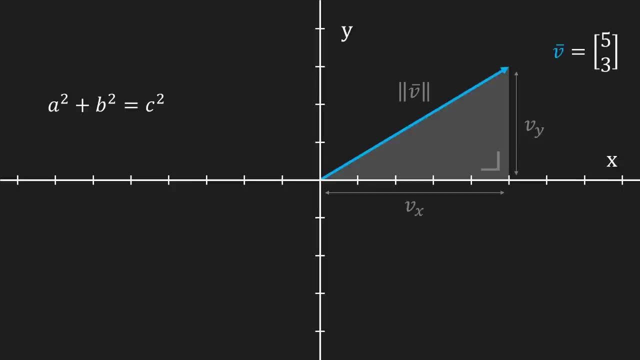 of a right-angled triangle, and c is the length of its hypotenuse. 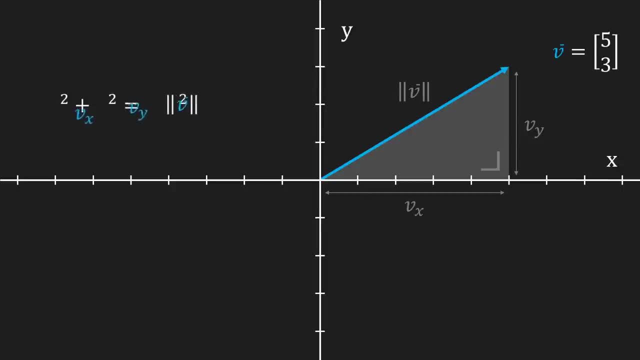 We can now replace a, b, and c with our vector's components. We can now replace a, b, and c with our vector's components. We can now replace a, b, and c with our vector's components, and the vector's length. We'll swap the left and right side of that equation, we'll take the square root of either side of the equation, and now we've got our expression for the length of a two-dimensional vector. 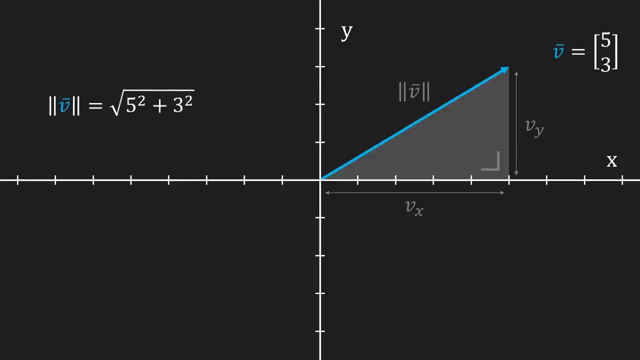 If we fill in the components of that vector in this case, we can calculate that this vector's 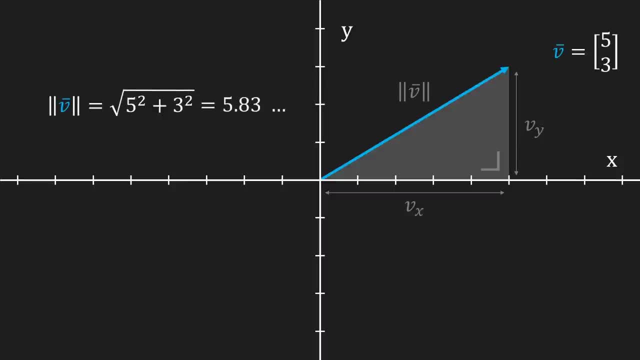 length is equal to 5.83 and a bit. 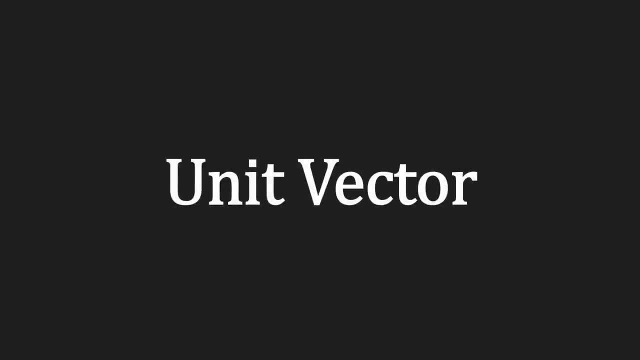 Concerning a vector's length, there is a special case which we call a unit vector. It's also referred to as a normalized vector. A normalized vector is a vector with a hat on top of it, and a normalized or unit vector is nothing more than a vector with a length of 1. In fact, we can take any arbitrary vector, divide it by its length, and then the result will be a vector that points in the same direction as the original vector, but that has a length of 1. 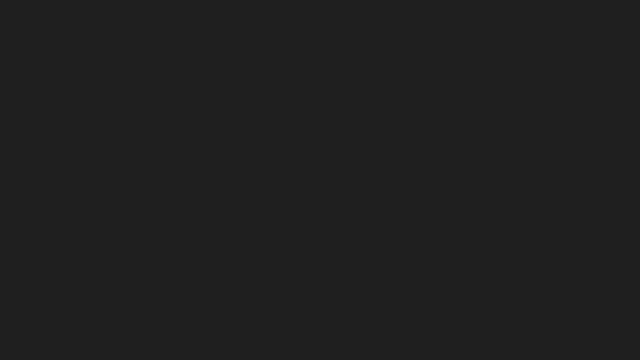 We also define a few standard unit vectors, being e hat x, which is a unit vector along the x-axis. e hat y, which is a unit vector along the y-axis. e hat y, which is a unit vector along the y-axis. 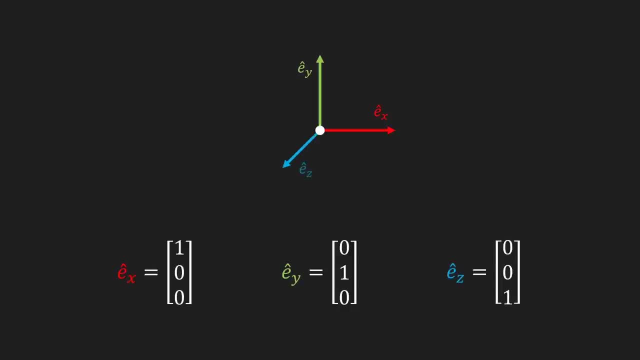 e hat z, which is a unit vector along the z-axis. Using these unit vectors, we can introduce an alternative way to write vectors, and that is to write them as the sum of their components multiplied by the respective unit vector. 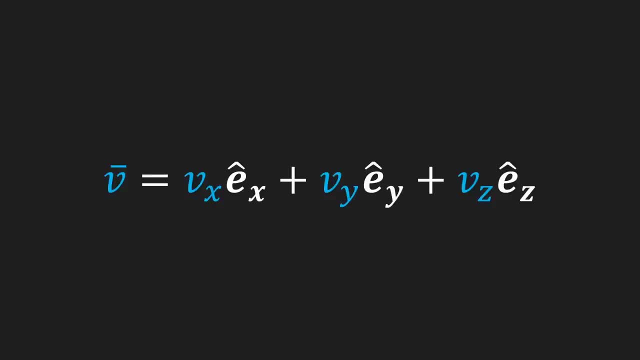 We call this unit vector notation, and we'll need it in just a bit. But first, we're going to discuss two ways in which we can multiply vectors. 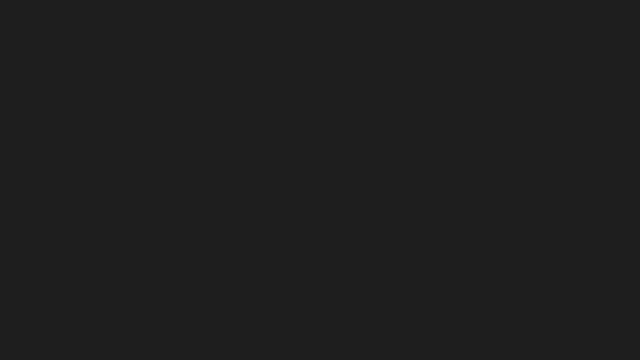 of 1.. We also define a few standard unit vectors, being e hat x, which is a unit vector along the x-axis, e hat y, which is a unit vector along the y-axis, e hat y, which is a unit vector along the y-axis. 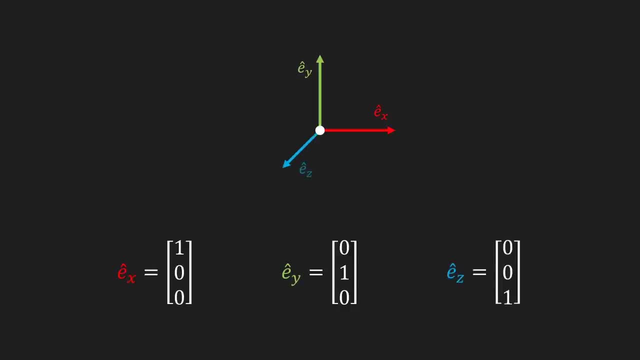 e hat z, which is a unit vector along the z-axis. Using these unit vectors, we can introduce an alternative way to write vectors, and that is to write them as the sum of their components multiplied by the respective unit vector. We call this unit vector notation, and we'll need it in just a bit. 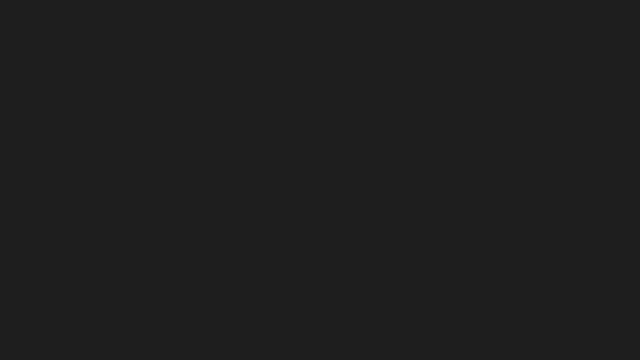 But first we're going to discuss two ways in which we can multiply vectors, The first one being the dot product, also referred to as the scalar product because its result is a scalar. We write the dot product of two vectors as a dot b, and in two dimensions it is defined. 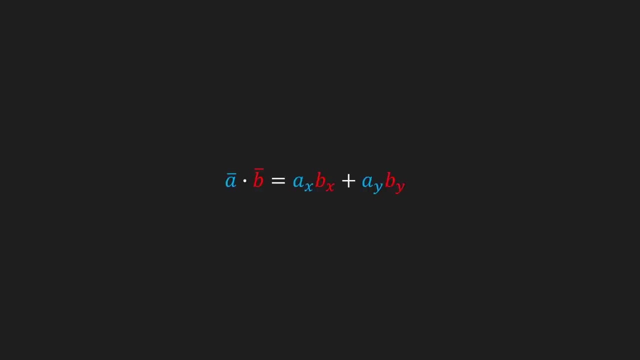 using this formula. We can extend this formula to three dimensions and, just like with a vector's length, we can also write a generic version for n-dimensional vectors. To understand the dot product, I'm going to draw a vector a and a vector b. I'll then. 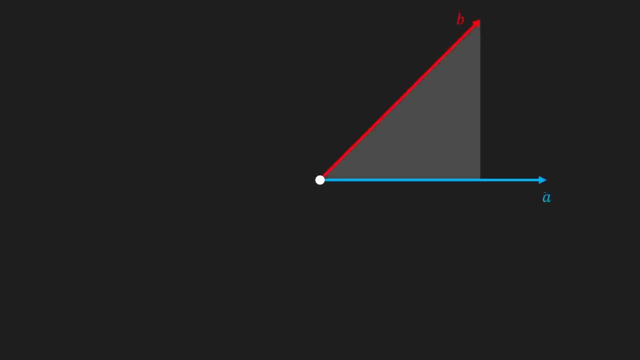 draw a triangle beneath vector b, So once again, this is a right-angled triangle. The dot product of a and b is now equal to the width of this triangle. However, there is a catch, and that is that I'm assuming that vector a is a unit vector. 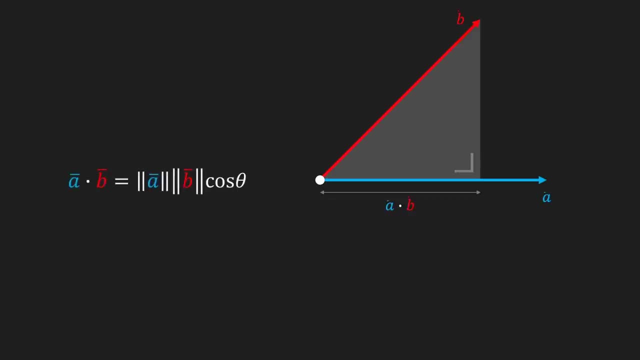 To explain this further, I'm going to introduce this alternative formula, which says that the dot product of vector a and b is equal to the length of vector a times the length of vector b, times the cosine of theta. Here, theta is the angle between vector a and b. 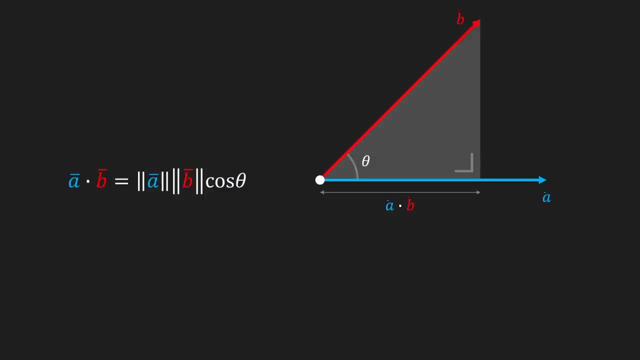 According to this formula, the dot product will get smaller if vector b gets shorter. It will get larger if the angle between a and b gets smaller. And finally, here's the catch, I've been assuming that vector a is a unit vector, because if 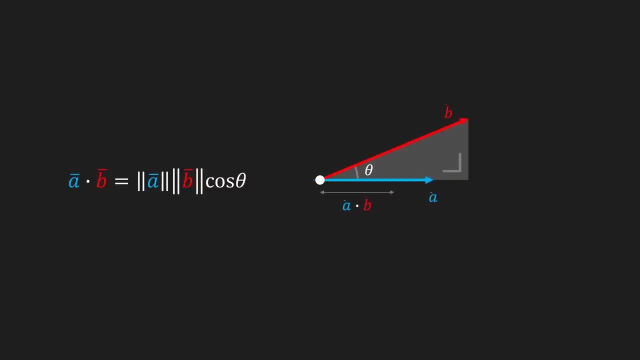 it's not. then the dot product will also be scaled by vector a and it will no longer be the width of our triangle. To dive a bit deeper into how the dot product changes based on the angle between vector a and b, I'm going to draw vector a and vector b and write our angle next to it. 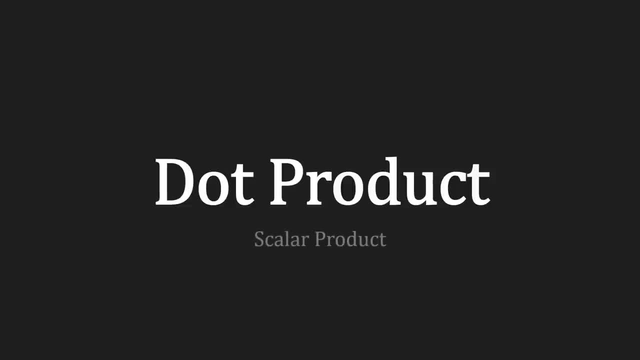 The first one being the dot product, also referred to as the scalar product because 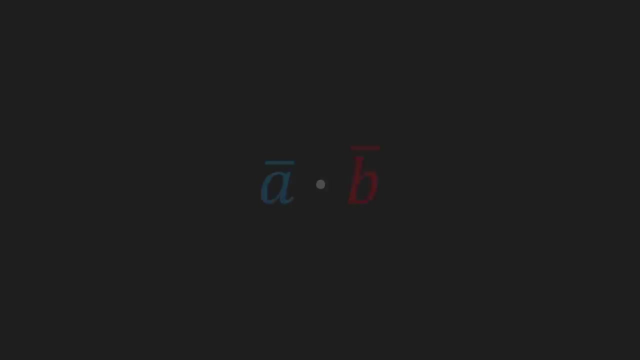 its result is a scalar. We write the dot product of two vectors as a dot b, and in two dimensions, it is defined using this formula. 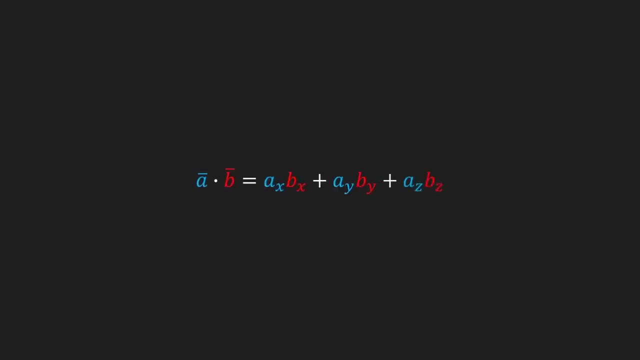 We can extend this formula to three dimensions, and just like with a vector's length, we can also write a generic version for n-dimensional vectors. 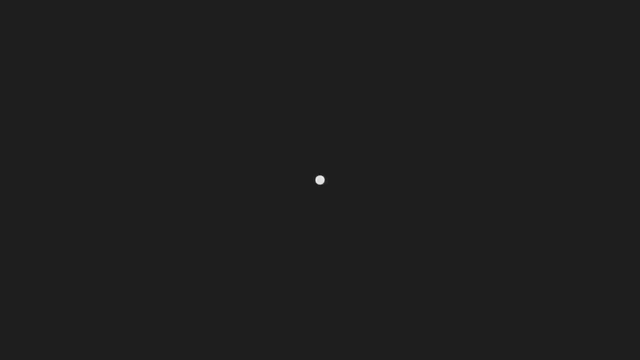 To understand the dot product, I'm going to draw a vector a and a vector b. I'll then draw a triangle beneath vector b, like this. I'll then draw a triangle beneath vector b, like this. I'll then draw a triangle beneath vector b, like this. 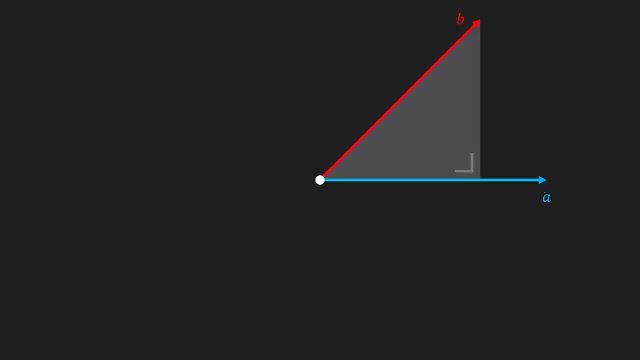 And once again, this is a right-angled triangle. 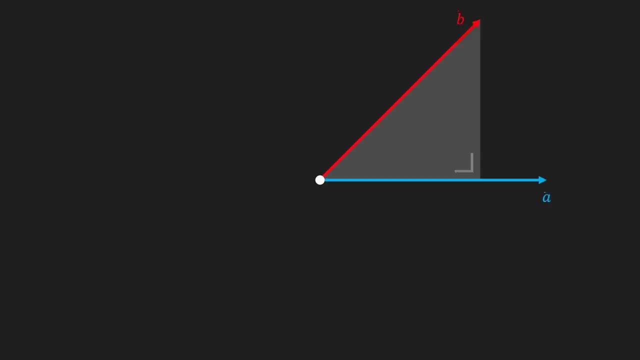 The dot product of a and b is now equal to the width of this triangle. 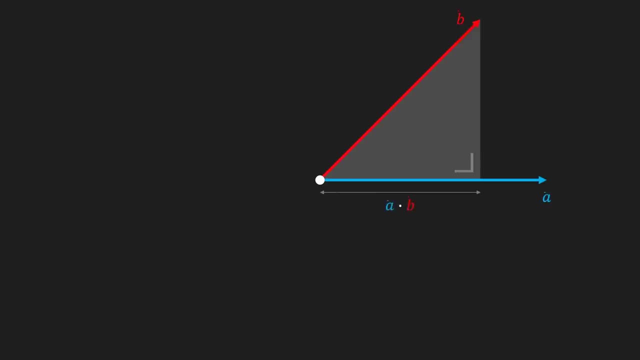 However, there is a catch, and that is that I'm assuming that vector a is a unit vector. To explain this further, I'm going to introduce this alternative formula, which says that 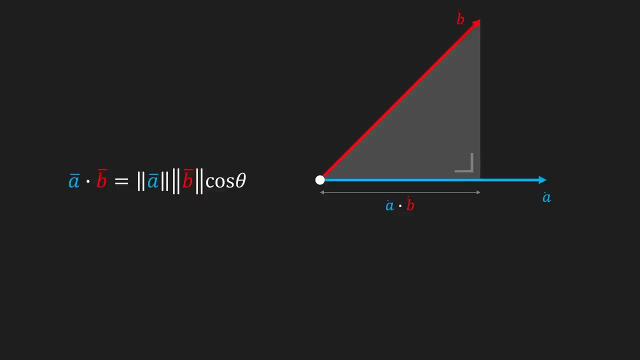 the dot product of vector a and b is equal to the length of vector a times the length of vector b times the cosine of theta. where theta is the angle between vector A and B. 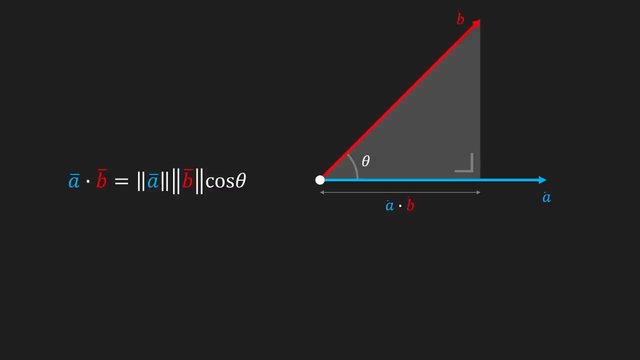 According to this formula, the dot product will get smaller if vector B gets shorter. 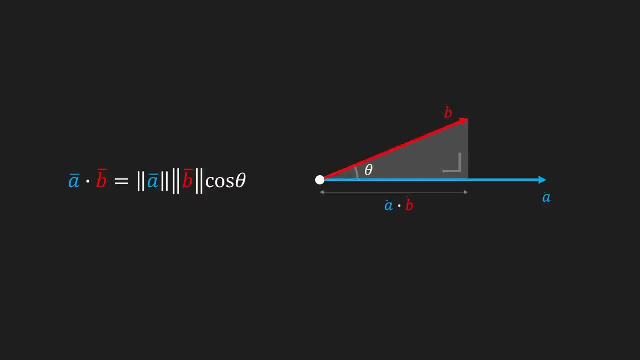 It will get larger if the angle between A and B gets smaller. 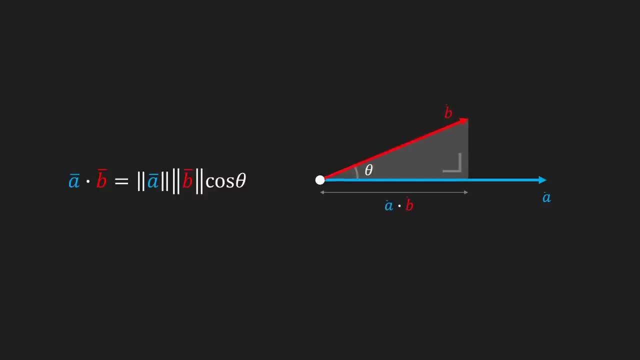 And finally, here's the catch, I've been assuming that vector A is a unit vector, because if it's not, then the dot product will also be scaled by vector A, and it will no longer be the width of our triangle. 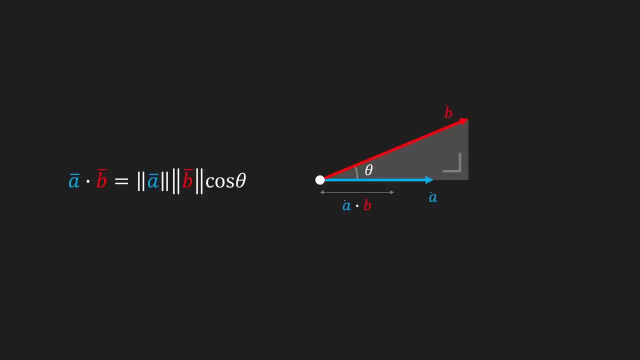 To dive a bit deeper into how the dot product changes based on the angle between vector A and B, I'm going to draw vector A and vector B, and write our angle next to it. If the angle between vector A and B is 0 degrees, 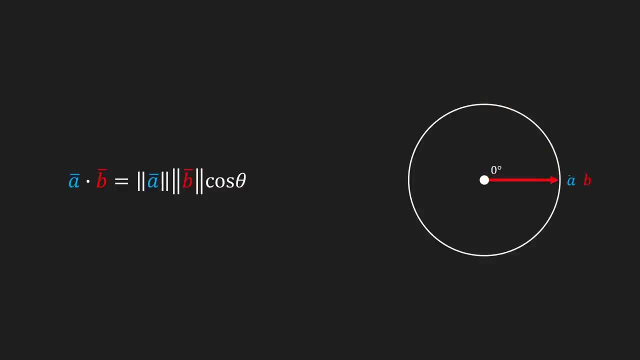 If the angle between vector a and b is 0 degrees, then the cosine of the angle between them, which is 0 degrees, will be equal to 1.. This means we can simplify our formula in the case that theta is 0 degrees, because 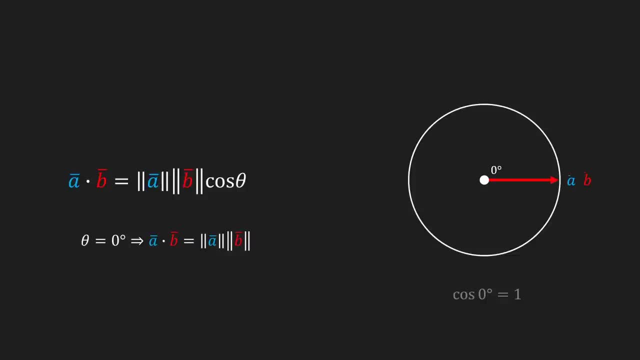 then the dot product of a and b is just the product- Thank you for watching this video- product of their lengths. Alternatively, if the angle between A and B is 90 degrees, or if it is 270 degrees, then the cosine of that angle will be equal to 0, and therefore we 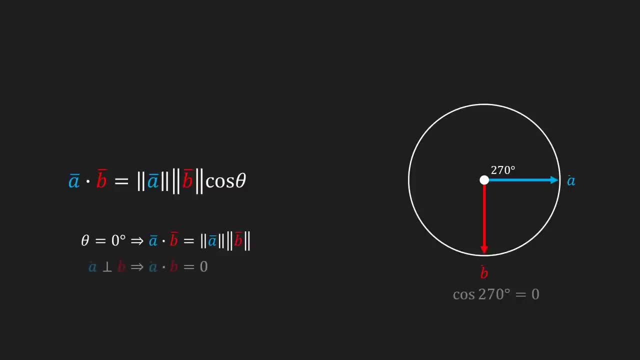 can once again simplify our formula for the dot product by saying that if A and B are perpendicular to each other, then their dot product will be equal to 0.. Finally, if the angle between A and B is 180 degrees, then the cosine of that angle is going to be equal. 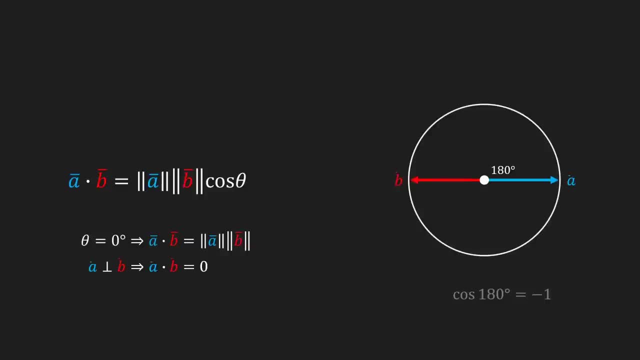 to negative 1, and then the dot product of vector A and B is going to be equal to the opposite of the lengths of A and B multiplied. We can simplify all these formulas even further if we assume that vector A and B are unit vectors. 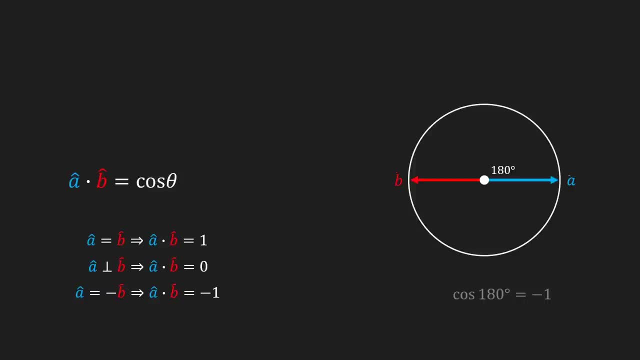 Out of this we can conclude that the dot product is equal to 1 if both vectors point in the same direction, that it is equal to 0 if both vectors are perpendicular to each other, and that it is equal to negative 1 if the vectors are opposite. In other words, 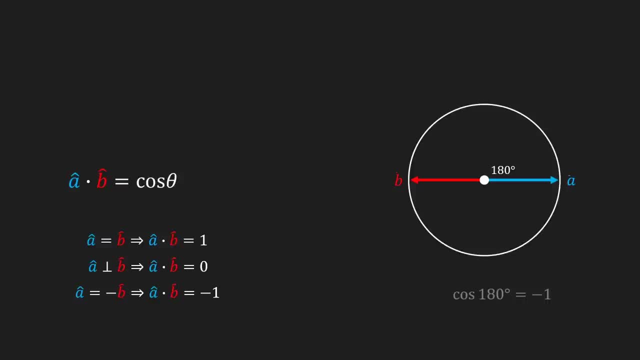 you can think of the dot product as a measurement for how similar two vectors are. I'm quickly going to come back to the original formula for our dot product, because if we reformulate that a bit, then we can write an expression to calculate theta, which was: 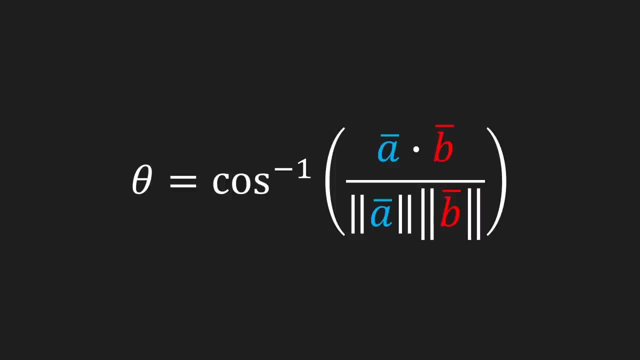 of course, the angle between A and B. There's one last thing about the dot product I wanted to show you, which is that the length of a vector is actually equal to the square root of the dot product of a vector itself. I'll leave that up to you to figure out why that is. 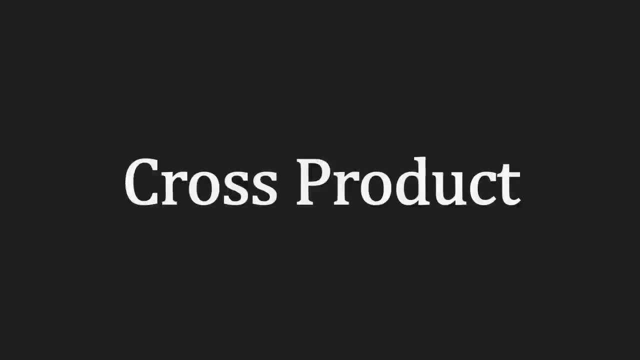 Let's now move on to that other way to multiply two vectors, which is the cross product, also referred to as the vector product. because the result is a vector, We write it as A, cross, B and it is defined as the determinant of the vector product. 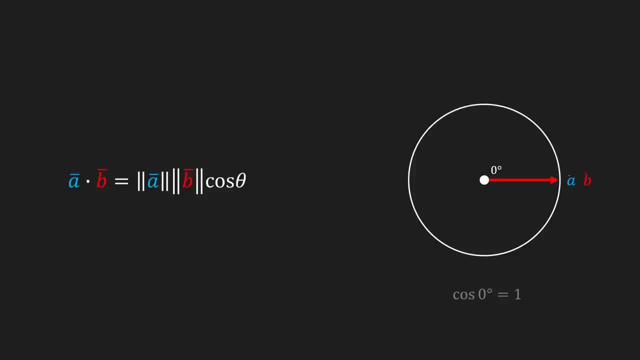 then the cosine of that angle between them, which is 0 degrees, will be equal to 1. This means that we can simplify our formula in the case that theta is 0 degrees, because then the dot product of A and B is just a product of their lengths. 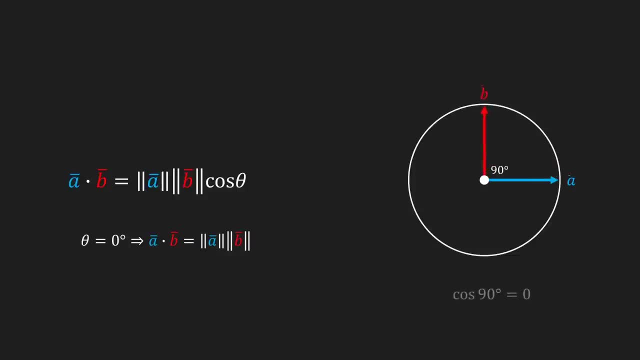 Alternatively, if the angle between A and B is 90 degrees, or if it is 270 degrees, then the cosine of that angle will be equal to 0, and therefore we can once again simplify our formula for the dot product, by saying that if A and B are perpendicular to each other, then their dot product will be equal to 0. 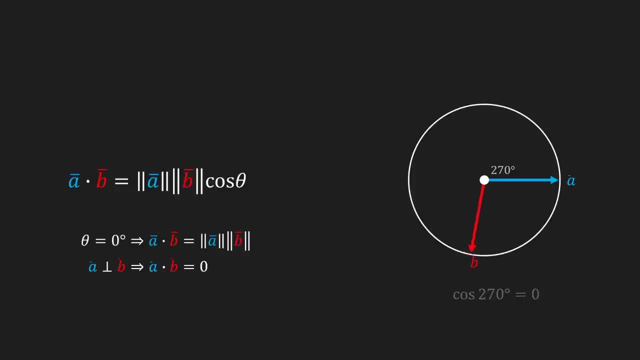 Finally, if the angle between A and B is 180 degrees, then the cosine of that angle will be equal to 0. If the angle between A and B is 180 degrees, then the cosine of that angle is going to be equal to negative 1, and then the dot product of vector A and B 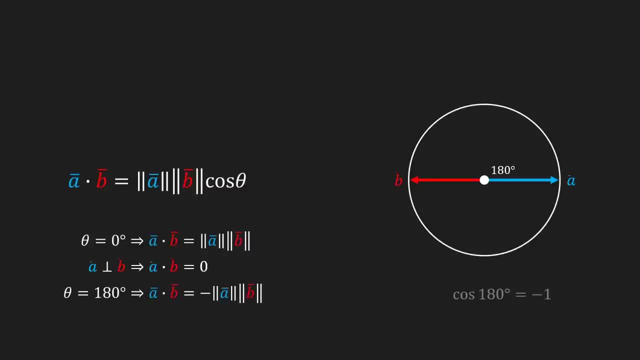 is going to be equal to the opposite of the lengths of A and B multiplied. 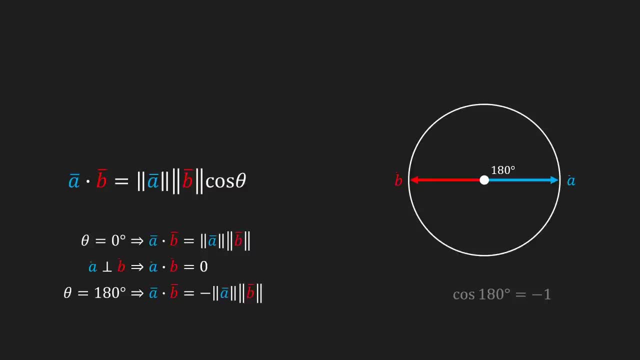 We can simplify all these formulas even further if we assume that vector A and B are unit vectors. Out of this, we can conclude that the dot product is equal to 1 if both vectors point in the same direction, that it is equal to 0 if both vectors point in the same direction, that it is equal to 0 if both vectors point in the same direction, if both vectors are perpendicular to each other, and that it is equal to negative 1 if the vectors are opposite. In other words, you can think of the dot product as a measurement for how similar two vectors are. I'm quickly going to come back to the original formula for our dot product, because if we reformulate that a bit, then we can write an expression to calculate theta, which was of course the angle between vector A and B. 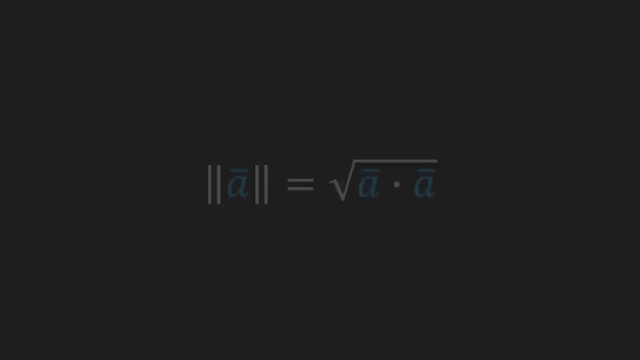 There's one last thing about dot product, I wanted to show you, which is that the length of a vector is actually equal to the square root of the dot product of a vector itself. I'll leave that up to you to figure out why that is. 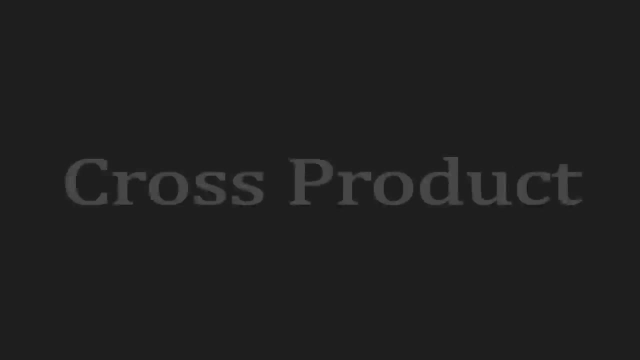 Let's now move on to that other way to multiply two vectors, which is the cross product, also referred to as the vector product because the result is a vector. We write it as A cross B, and it is defined as the determinant of this matrix. 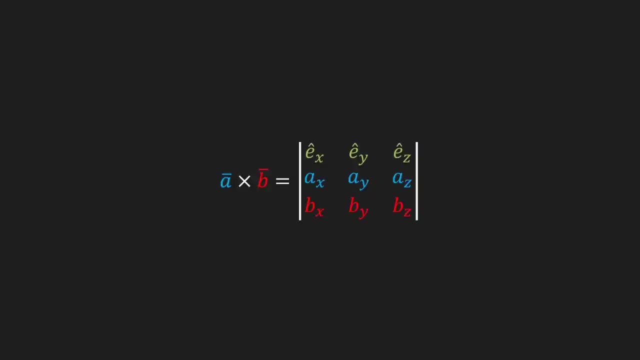 The vector product is a vector and it is defined as the determinant of the vector product, and it is defined as the determinant of the vector product. Now, we haven't covered matrices yet, leave alone how to calculate their determinant. so you just have to take from me that that result is equal to this massive formula. 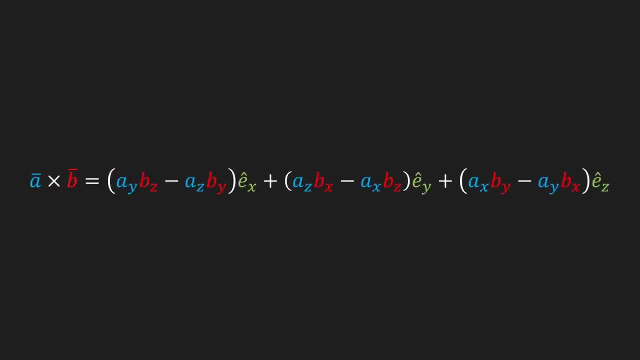 However, if you take a closer look at this, you might recognize unit vector notation, which means that we can actually rewrite this formula between our beloved square brackets. Also, notice that the cross product is only defined in three dimensions. To visualize what the cross product means, I'm gonna once again draw vector A and vector. 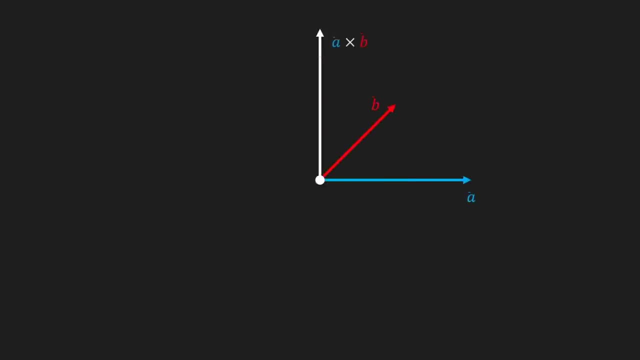 B. Their cross product is equal to this white vector, Unlike the dot product. the order in which you take the cross product of two vectors actually matters, because if you take the cross product of B and A, you get a vector that points in the opposite direction. 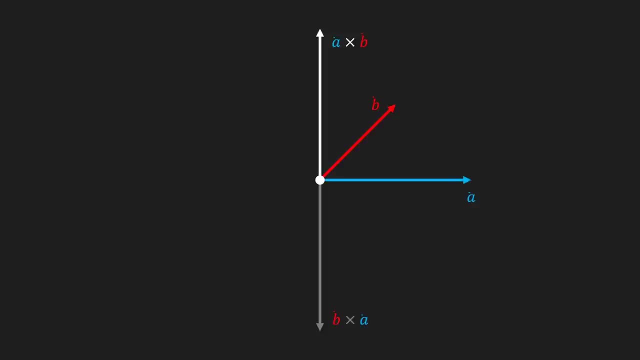 So you could therefore say that the cross product of B and A is equal to the opposite of the cross product of A and B. The cross product results in a vector that is perpendicular to the original vectors. You can visualize this using the right hand rule. 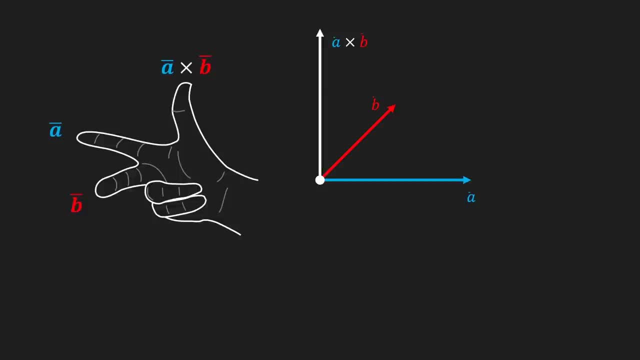 If you take your right hand and point your index finger in the direction of vector A, your middle finger in the direction of vector B, then your thumb will point in the direction of their cross product To show some of the properties of the cross product. I'm gonna introduce this alternative. 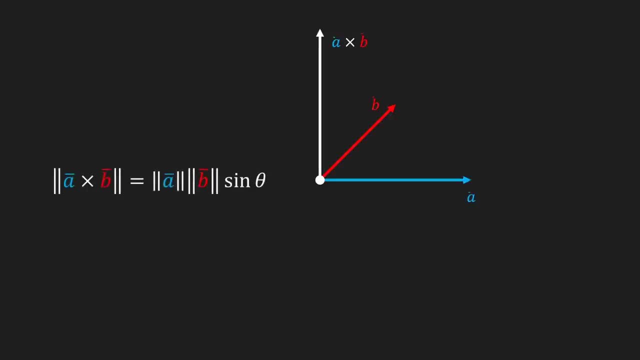 formula that says that the length of the cross product of vector A and B is equal to the length of vector A times the length of vector B times the sine of theta, and theta is once again the angle between vector A and B. Another way to think of the length of the cross product of A and B is to think of it. 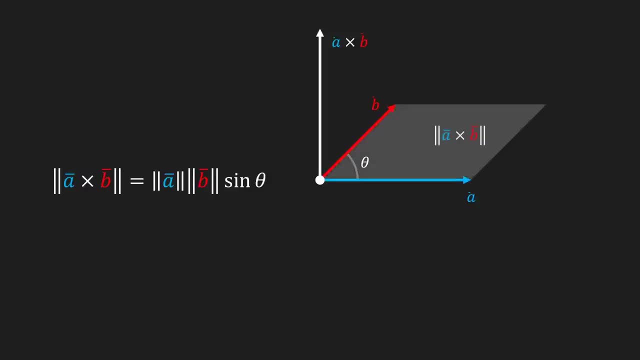 as the area of the parallelogram between vector A and B. According to this formula, the length of the cross product will become shorter if vector A or B get shorter. Moreover, if the angle between A and B gets smaller. To show why that is, I'm gonna draw once again vector A and B and I'm gonna display the 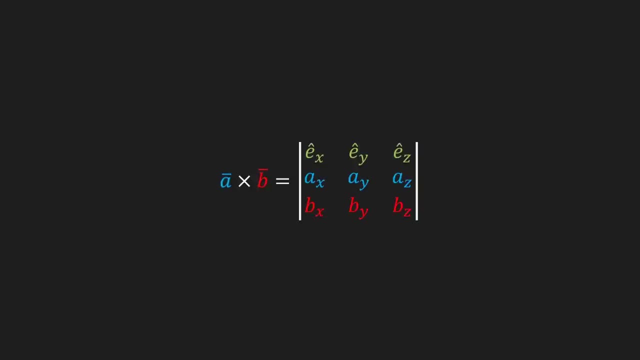 Now, we haven't covered this, we haven't covered matrices yet, leave alone how to calculate their determinant, so you just have to take from me that that result is equal to this massive formula. 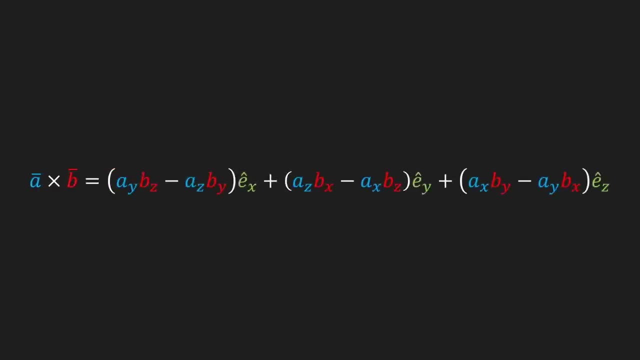 However, if you take a closer look at this, you might recognize unit vector notation, which means that we can actually rewrite this formula between our beloved square brackets. Also notice that the cross product is only defined in three dimensions. To visualize what the cross product means, 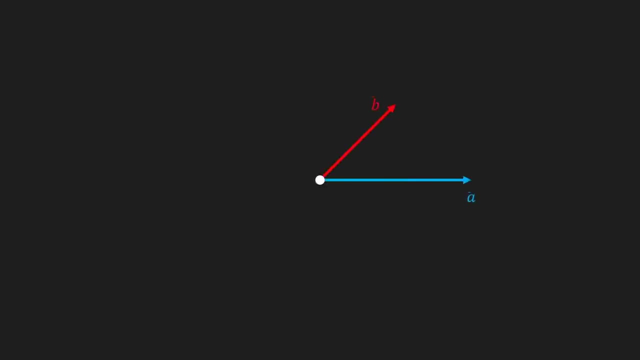 I'm going to once again draw vector A and vector B. Their cross product is equal to this white vector. 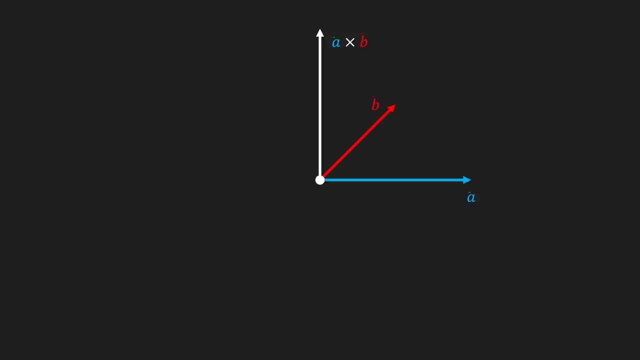 Unlike the dot product, the order in which you take the cross product of two vectors actually matters, because if you take the cross product of B and A, you get a vector that points in the opposite direction. So you could therefore say that the cross product of B and A is equal to the opposite of the cross product of A and B. 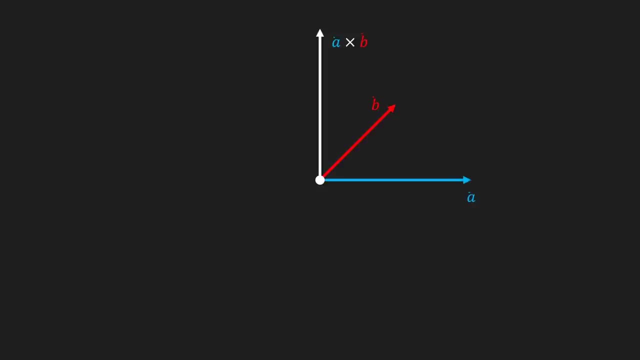 The cross product results in a vector, that is perpendicular to the original vectors. You can visualize this using the right hand rule. 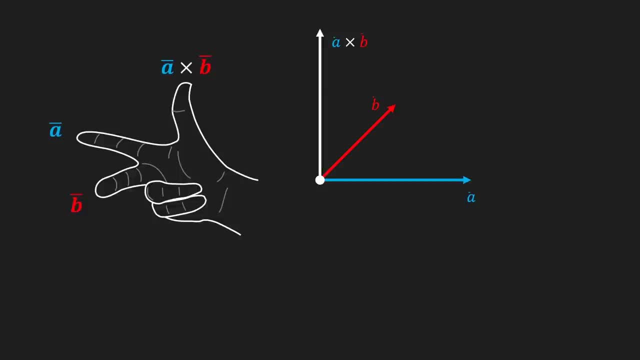 If you take your right hand and point your index finger in the direction of vector A, your middle finger in the direction of vector B, then your thumb will point in the direction of their cross product. 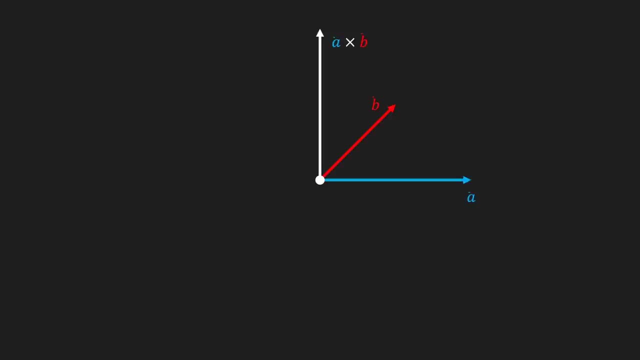 To show some of the properties of the cross product, I'm going to introduce this alternative formula, that says that the length of the cross product of vector A and B 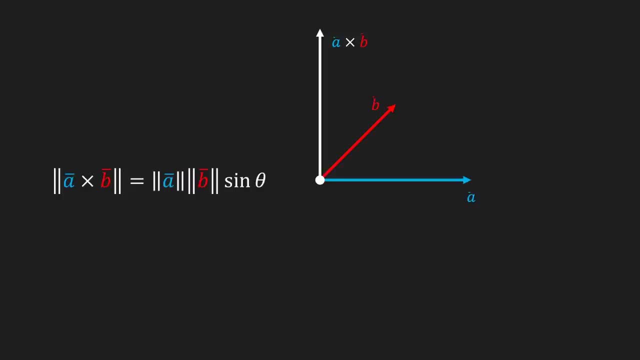 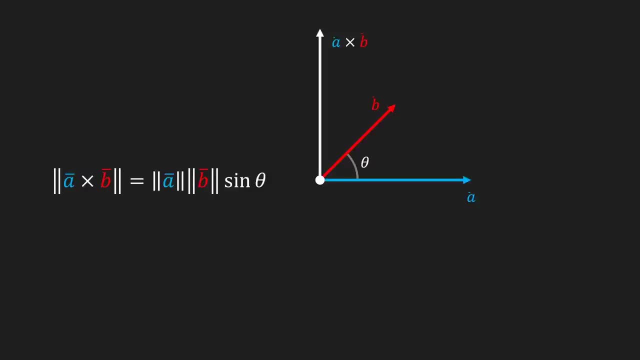 Another way to think of the length of the cross product of A and B is to think of it as the area of the parallelogram between vector A and B. 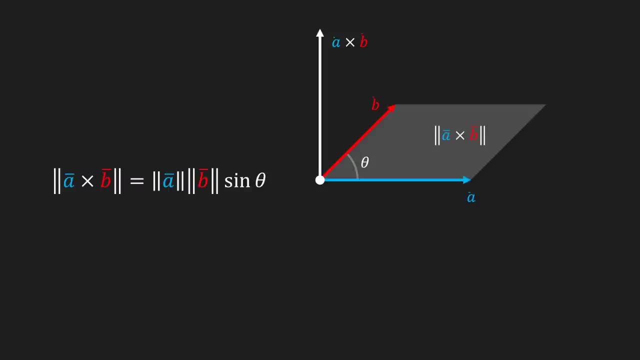 According to this formula, the length of the cross product will become shorter if vector A or B get shorter. 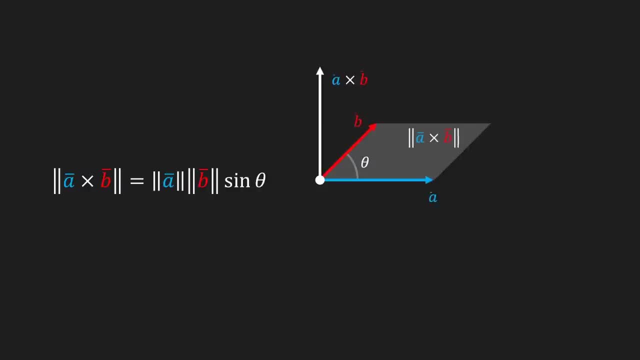 The cross product will also get shorter if the angle between A and B gets shorter. The cross product will also get shorter if the angle between A and B gets shorter. To show why that is I'm going to draw once again vector A and B